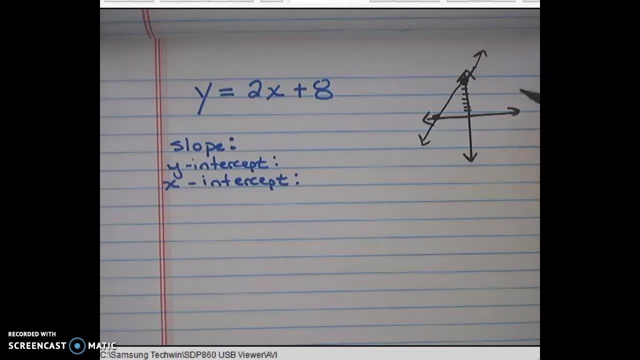 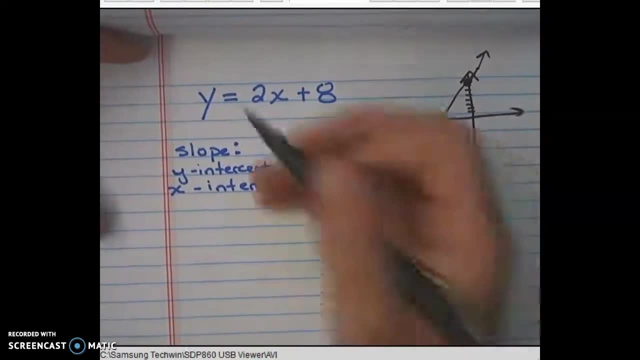 What we're going to look at today is: how can we just find it if we didn't have a graph? How does the equation tell me that information? so I don't need to graph it. So we already talked about two things. Because this is written in: y equals mx plus b. 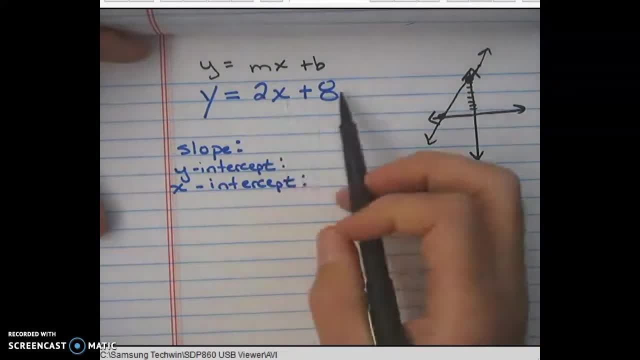 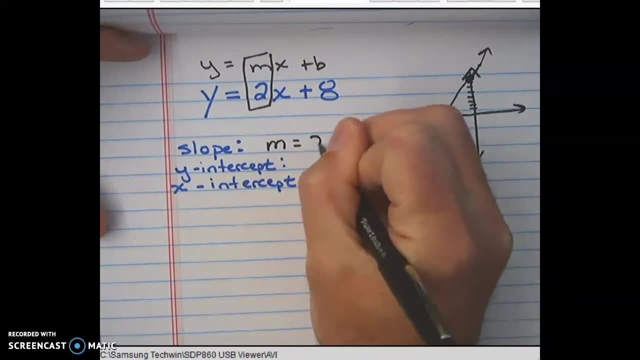 slope-intercept form tells us two things. just by looking at the equation, It tells us the slope is 2.. So here, where it says slope, you could say the slope is equal to 2.. And it also tells us our b, which stands for the y-intercept. 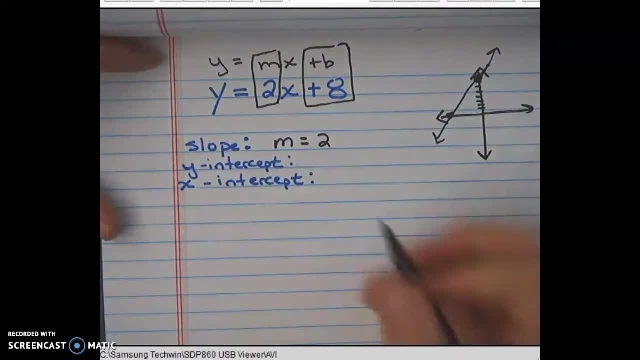 Now, when we talk about y-intercepts, we want to make sure we don't just write 8 for the y-intercept- Although if someone said the y-intercept is 8, we would probably all know what they're talking about. We like to write y-intercepts as points. 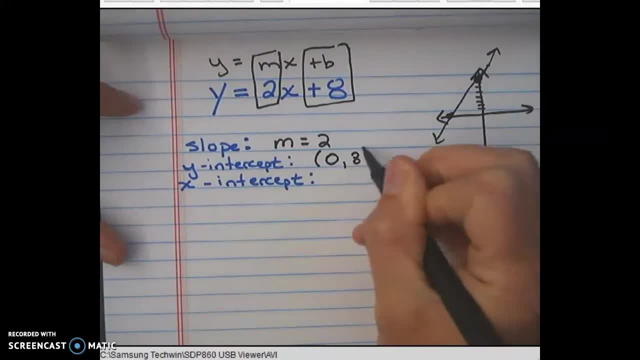 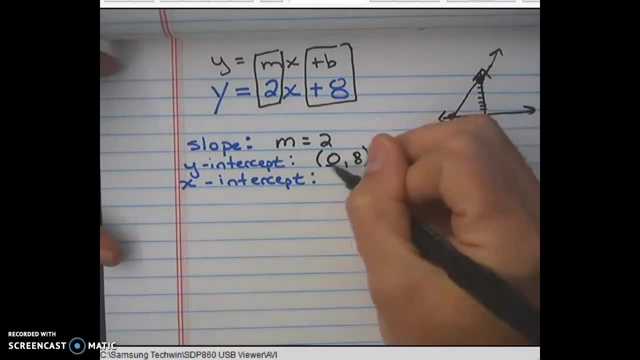 It's the point that's 0 over and 8 up, And so what we're going to talk about today, which is going to help us figure out our x-intercept, is this idea that the intercepts happen at either where x. 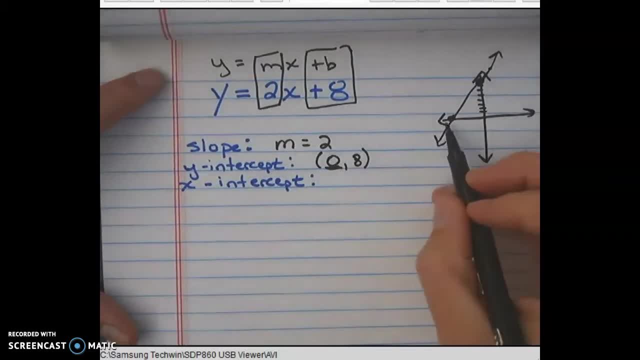 x is 0,, so up on the y-axis, or where y is 0,, somewhere on the x-axis, And so we could look at it graphically and also show that the y-intercept is 8.. If we didn't, sorry, not graphically, but algebraically. 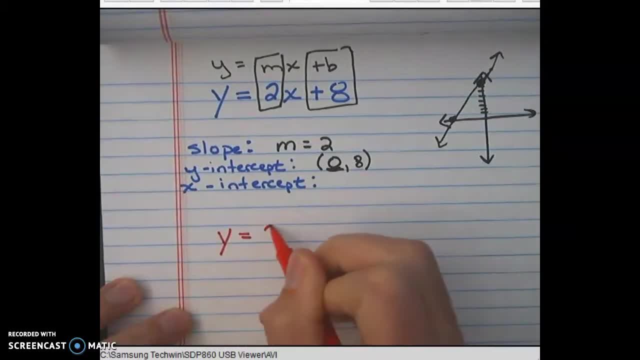 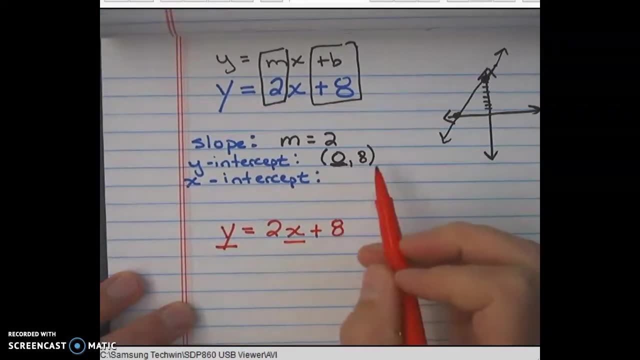 And that is by taking the equation y equals 2x plus 8, and just realizing that the x and the y are coordinate pairs that are all on this line. that would make up the y-intercept, And so we could look at it graphically and also show that the y-intercept is 8, if we didn't. sorry, not graphically, but algebraically. 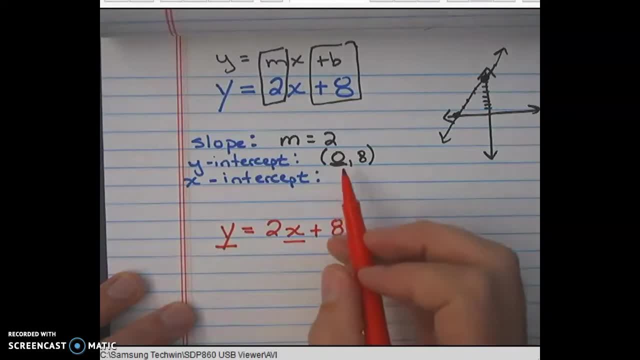 And so we could look at it graphically and also show that the x and the y are coordinate pairs that are all on this line. that would make up the y-intercept. And so if I know that my y-intercept that's the one that touches the y-axis. 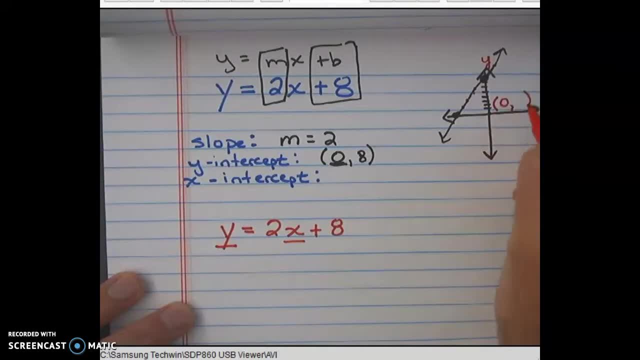 every point on the y-axis has an x value of 0, I can plug in 0 for my x and then figure out what the y-coordinate should be. So in this problem if I want to find the y-intercept, I know in y-intercepts the x value is 0,. 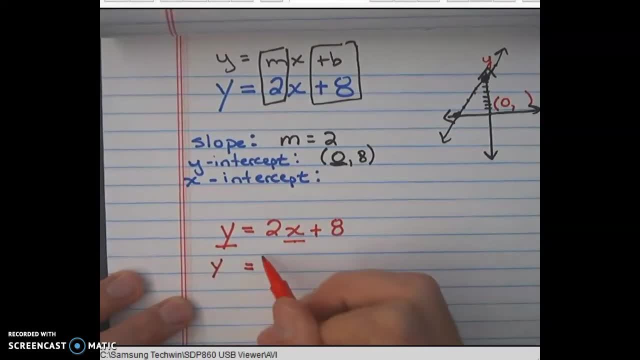 I could say: alright, my y value, which I don't know, is equal to 2 times my x value, so that's 0 plus 8.. And if I solved it- not really solved it, but just evaluated it- 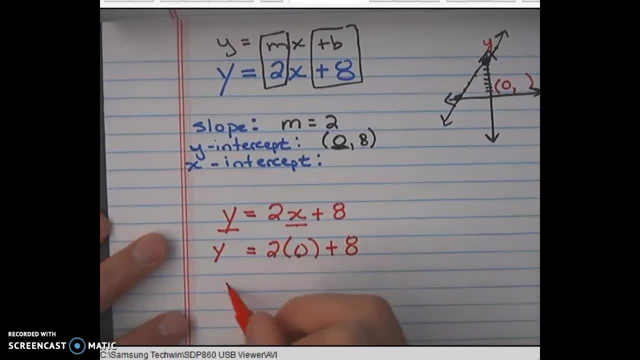 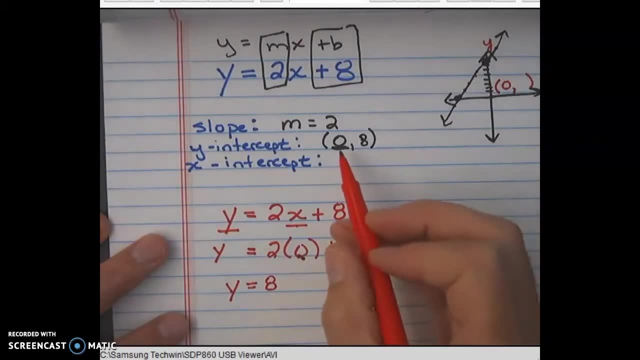 2 times 0 is 0, plus 8 is 8.. So the y-coordinate to this point is 8 when x is 0. That's why we get a y-intercept of 0, 8.. Now again, you probably wouldn't need to do this algebraic step. 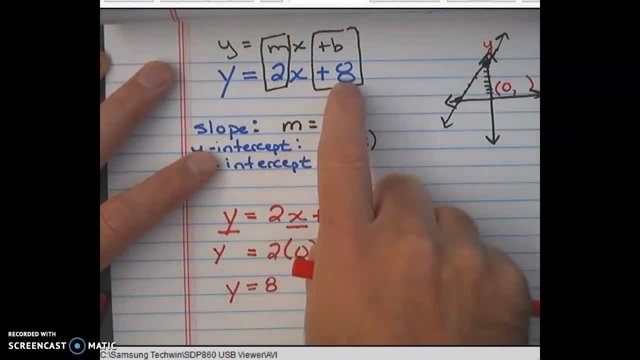 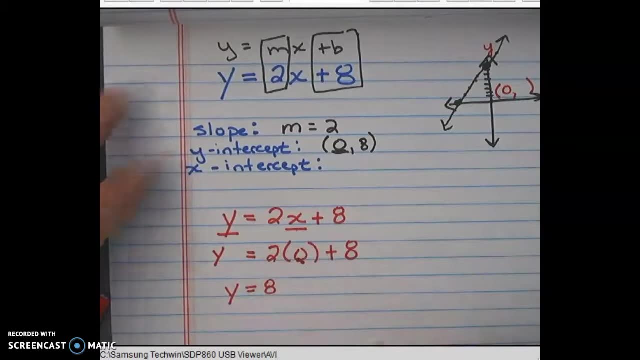 because if it's in slope-intercept form I know that number- that's by itself, without the x, is the y-intercept. so I could just write 0, 8 here. But this helps us start to understand how we find the x-intercept as well. 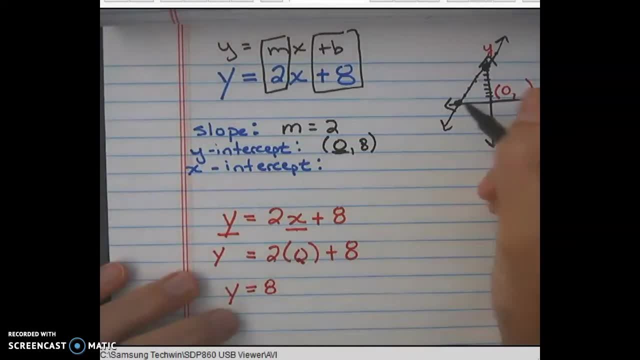 Because in the x-intercept, when it touches the x-axis, it's not that our x value is 0 anymore. we have an x value. We're over. it looks like it's going to be negative, something over, but we're 0 up. so now we know our y-value is 0.. 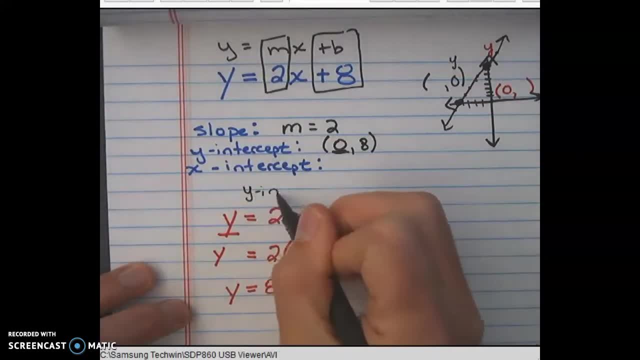 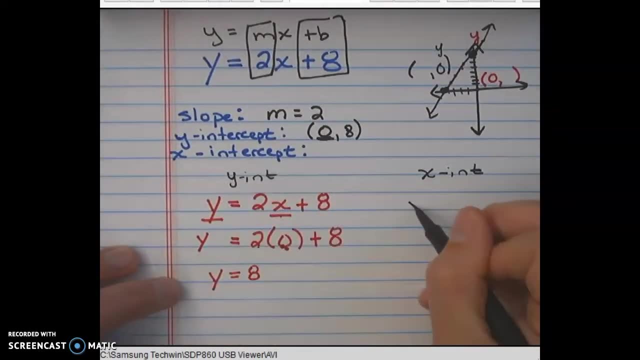 And so I could do the same thing. so this was to find the y-intercept. I can do this. I can do the same thing to find the x-intercept, But in the x-intercept, in y equals 2x plus 8,. 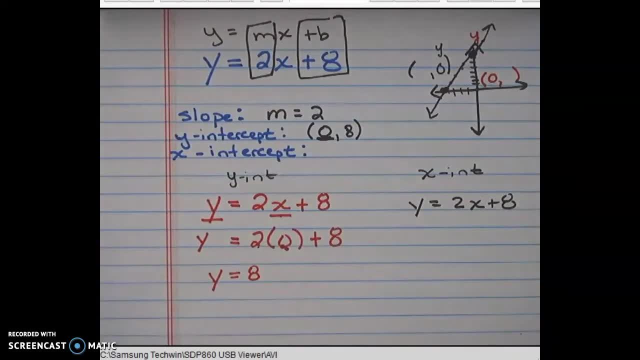 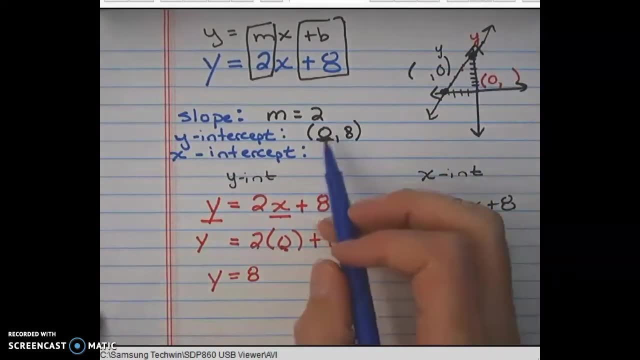 it's the y-value that's 0.. So this is the important part, Important enough that I'm going to say it again: In a y-intercept, when it crosses the y-axis, the x-value is 0.. It's kind of the opposite of what the words are. 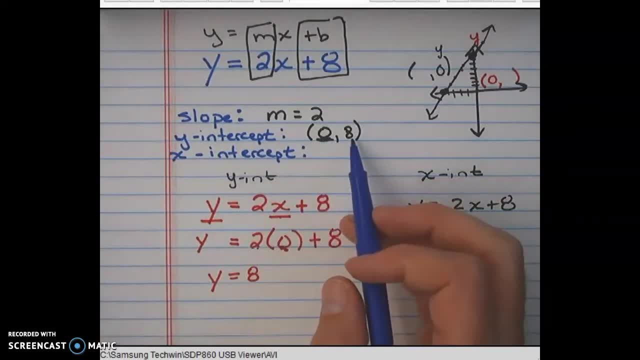 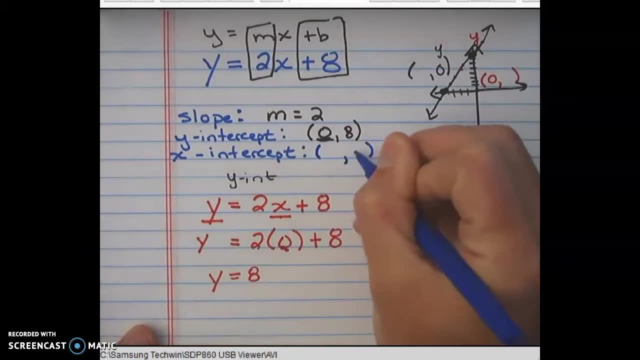 So in the y-intercept the x is 0, because we actually have a point on the y where it intercepts it. So in the y- Intercept it's going to be- I can think of my answer- it's going to be the y-value, that's 0.. 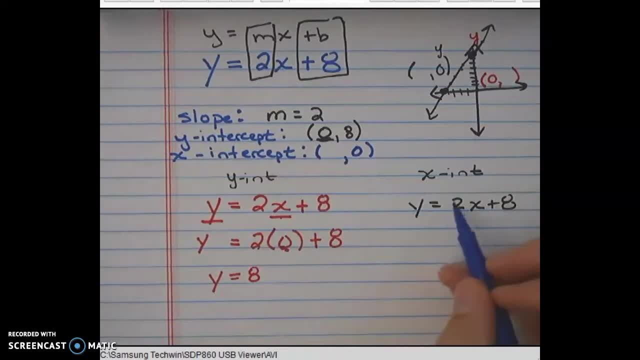 So when I go to plug in what I know into this equation- last time I plugged 0 into x because I was looking for a y-intercept. If I want to find a x-intercept, then I'm going to plug in 0 for y. 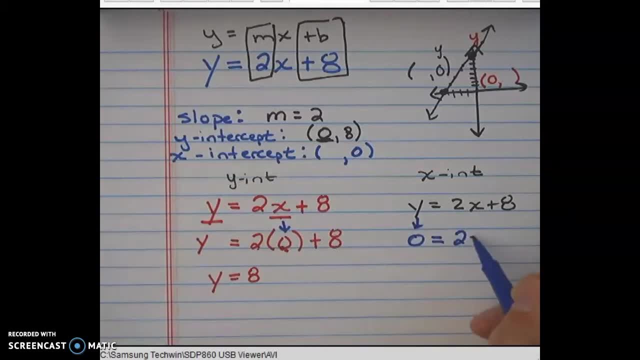 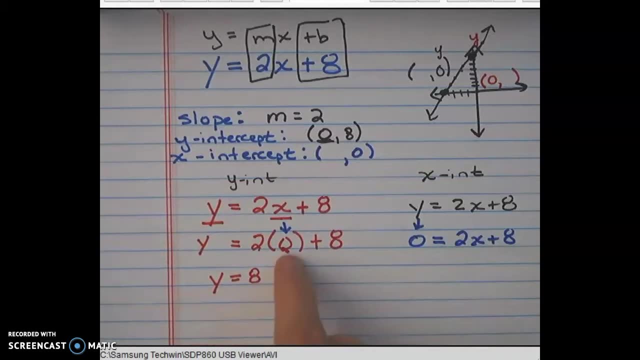 So instead of the y-value I'm going to plug in 0 and say 0 equals 2x plus 8.. And now I'm going to figure out what x is Now on this side. y was already by itself, so I just did all the math Here. x is not by. 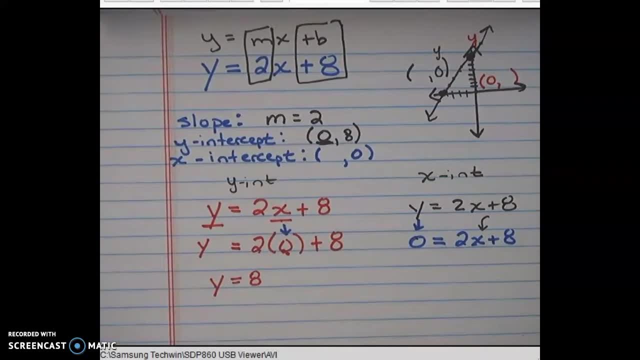 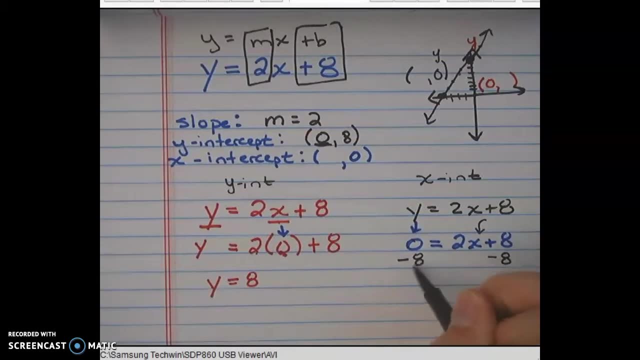 itself. so I have to solve for x. So I've got to do a little bit of solving. but that's fine. Start farthest away from the x to get x by itself, which is the plus 8.. So we subtract 8 from both sides.